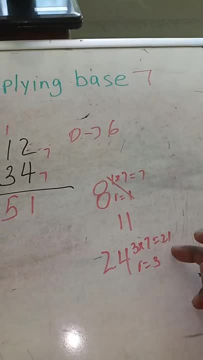 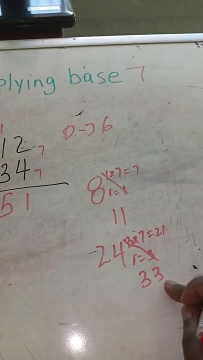 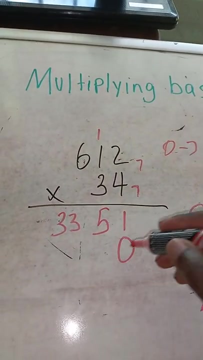 would be three, so the remainder would be 3. so we have three, three, seven, twenty one plus three, equal twenty four, three, three. all right, so four, six is twenty four, three, three, and we had a zero here because we're no longer deal with the ones column where no movement, intense column will put a 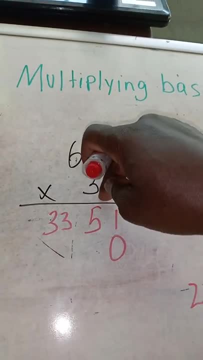 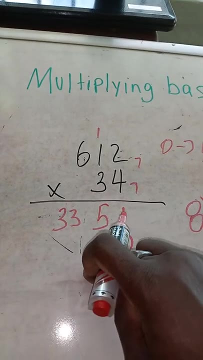 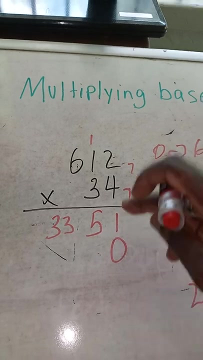 zero here, because the zero ten has one zero, so put a zero here. all right, if it was dealing with a hundred, over here is oranges column will put one, two zero, because a hundred has two zero. but we're dealing with ten, and ten has one zero, so put a zero here. and then we start here. three times two equals six. 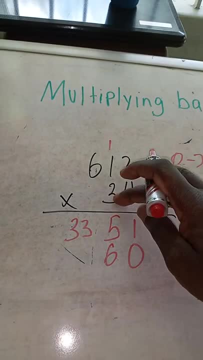 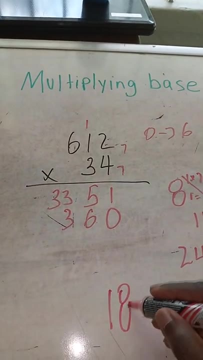 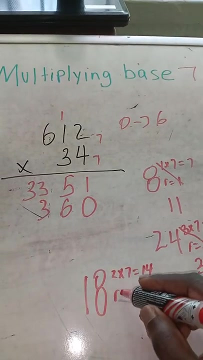 can we write six? yes, because six is lower than seven. three one, three equal three. three six is 18. can we write 18? no, we can't. over the time, can seven go into 18? let us try to: two times seven equal 14 and remainder is 14 from 18 leave. 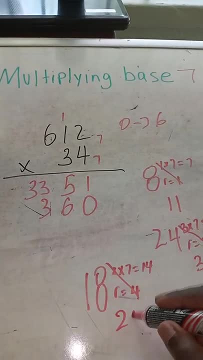 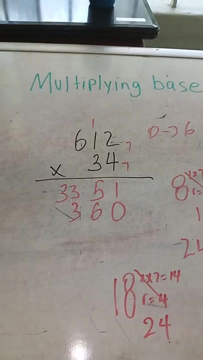 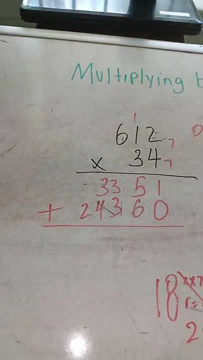 14, four. so the answer would be two, four. so this is what you used to represent: 18, two, seven, fourteen plus four equal 18. all right, so put the two, four there. we draw our line, we put our operation. we're no longer multiplying, we're no adding very. 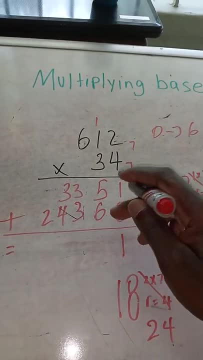 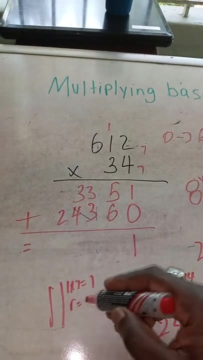 good, all right. so one times zero, one six and five equal 11. we can't write 11. one times seven equals seven. we can't write 11. we can't write 11. we can't write 11, so we need to get four equals seven. the remainder would be what mm. four, because 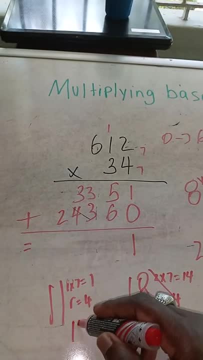 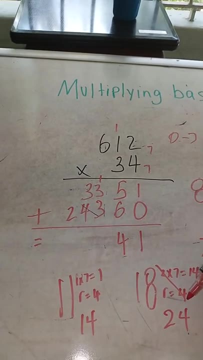 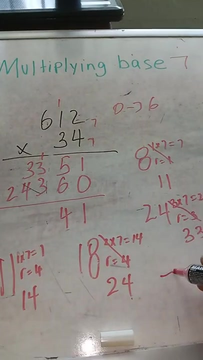 seven from 11 equal four and we have one four as representation for it. we put down the four and we carried one three, six and one seven. can we write 7? no, we can't write 7, remember the ice number we can write is 6. so one times 7 equal 7 and remainder equals 10.. pour into A play자 to make a colour nên you need to call and you will be finished there. for seven. two is arrived, appear again for three, four and the remainder will be one, seven, three, two a a half and 7 of 6, now initial, and we are going to give them a 7 here, 7 a 5.. In this case, this equation is 1,. 2 package has a 3, which means that you are going to be left behind, but the the meaning is first, and in frankly it's 4: 2 package. vice versa.